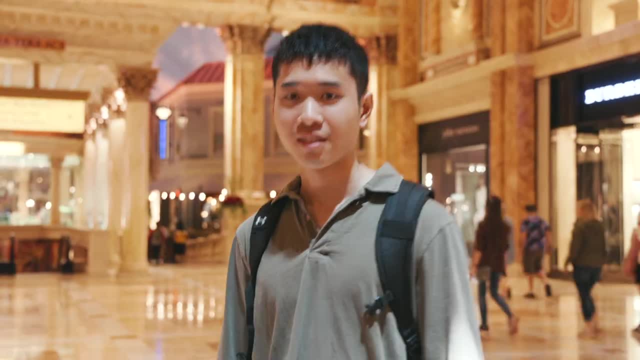 If you subscribe because of my travel content, stay tuned because there's so much more to come. This video is geared towards helping people navigate their career in data. I'm going to cover the why, share some useful resources and talk about the mindset in order for you to succeed. 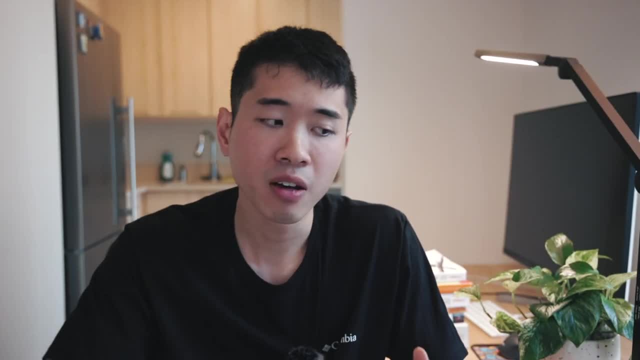 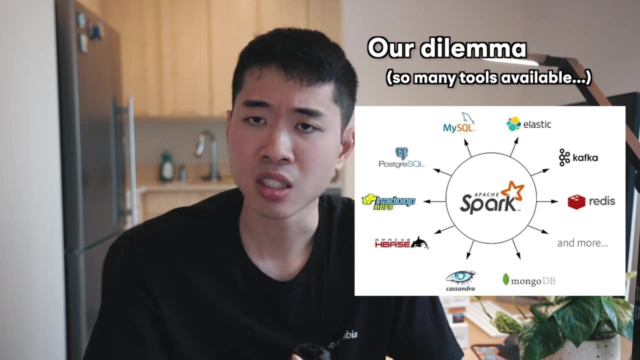 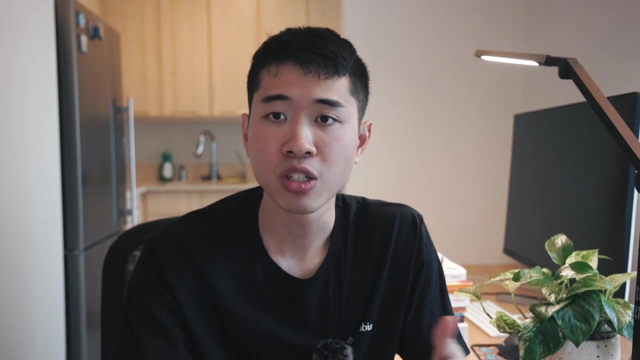 Let's dive right in. So when I was first starting out, I felt super overwhelmed because I kept seeing a lot of buzzwords on the internet. For example, what is Spark, Hadoop, Hive? Not only that, but data engineering is a lot more ambiguous compared to traditional tech roles like software. 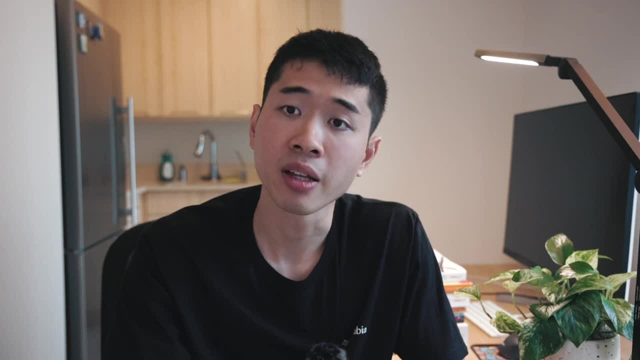 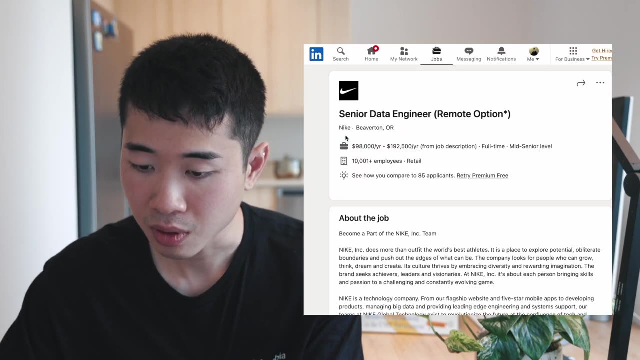 engineering. Let's take a look at an example job description on LinkedIn. All right, let's search data engineer, and well, this one looks good. Senior data engineer, Nike. Okay, if I scroll down to the job description, you'll see words like expertise with relational SQL. 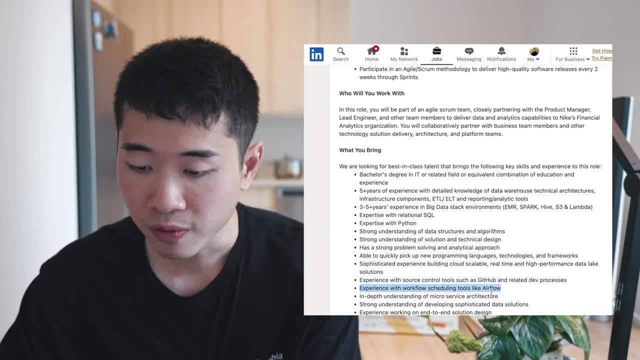 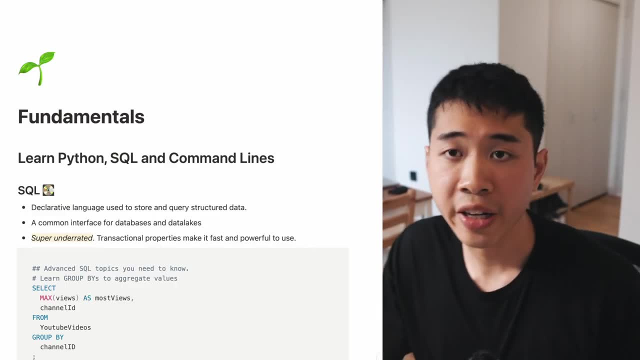 expertise with Python. experience with workflow scheduling tools like Airflow. When you're starting out, learn about Python, SQL and command lines. All your tools as a data engineer are going to have abstraction layers over these three things. Not only that, but you'll be interviewing using Python and SQL. 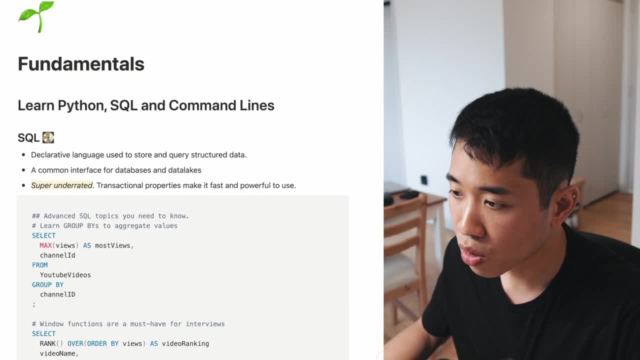 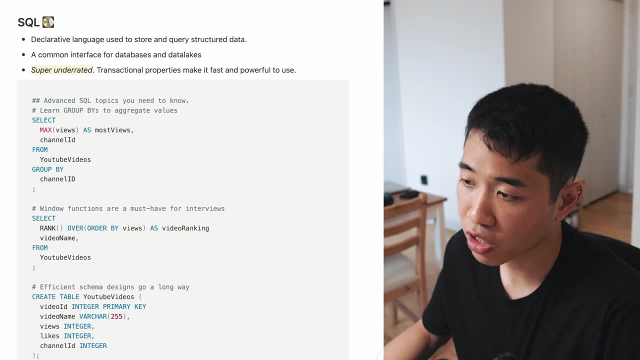 So most people know SQL as a declarative language used to store and query structured data. But what most people don't know is that SQL has a lot of attractive transactional properties that make it really fast and easy to use. SQL is super underrated. 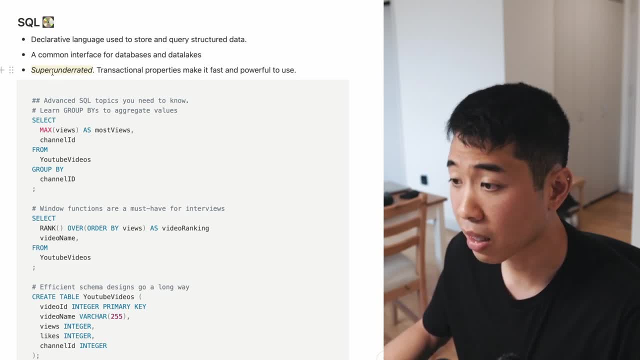 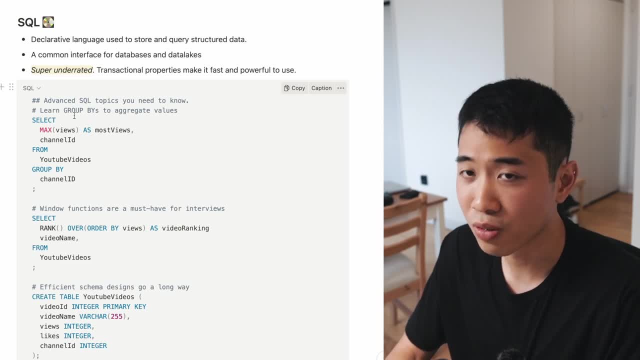 Every single YouTube video in the world and I want to find out what is the most viewed video per channel ID or the channel name. I can do that using group by functions, by using channel ID as my group, by key and taking the aggregate maximum value of views. Window functions are very similar. 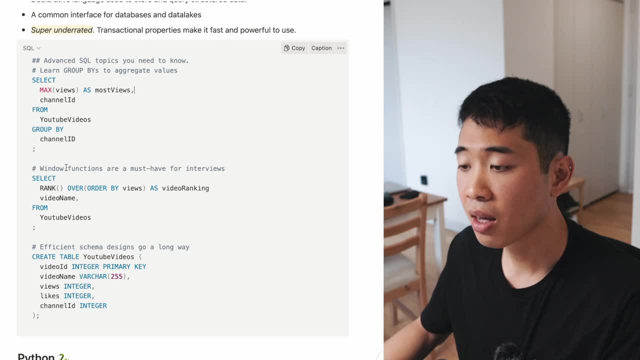 to group by functions. in the sense that they both aggregate values, They are a must have for interviews. I remember when I was applying for all these data engineering positions, I would constantly get thrown questions about window functions For programming languages. I wouldn't. 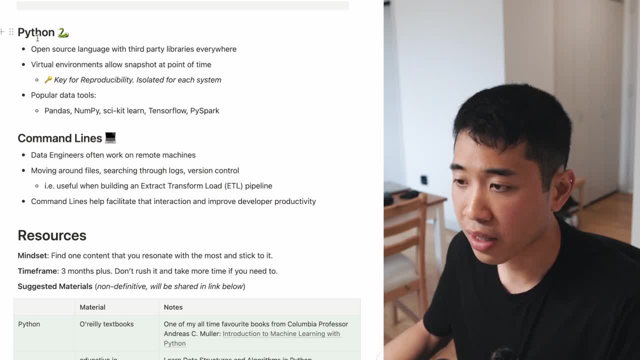 recommend starting out using Java or other object oriented languages, because the objective is to learn about data concepts, not computer science. Python is an open source language with a bunch of third party libraries. everywhere. We have something called virtual environments which allow us to store snapshots of your system at a point of time. This is really key for reproducibility, where we 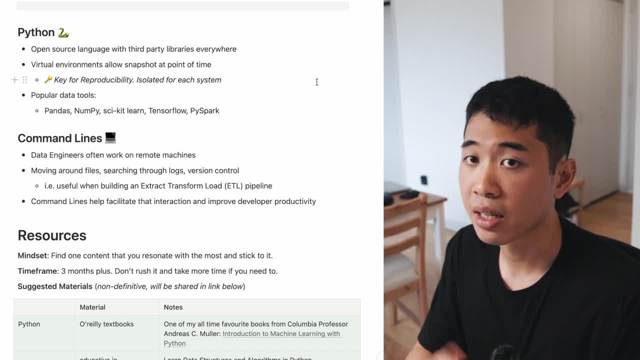 want to build data engineering systems that are isolated against each other. For command lines, let's say we're building a data pipeline that move around files, search through logs. Command lines help facilitate that interaction and help data engineers be more productive. Here are some. 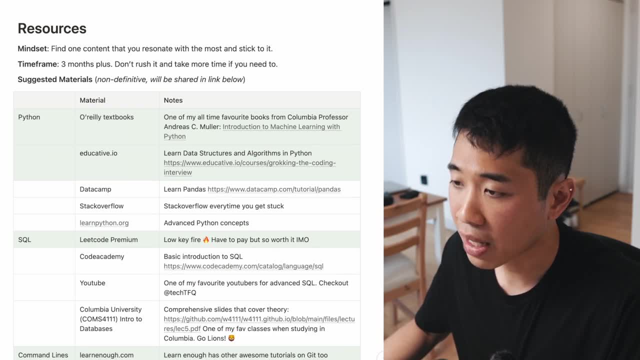 useful resources. I will give myself three months plus, and don't rush it. Take more time if you need to. The mindset here is that you should find one content that you resonate with the most and just stick to it. I've listed down a few of the most popular ones. I've listed down a few of the most. 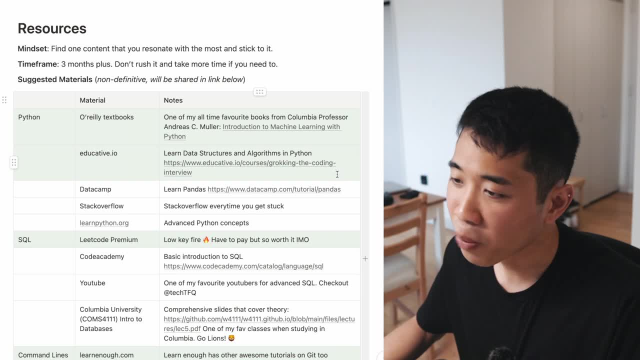 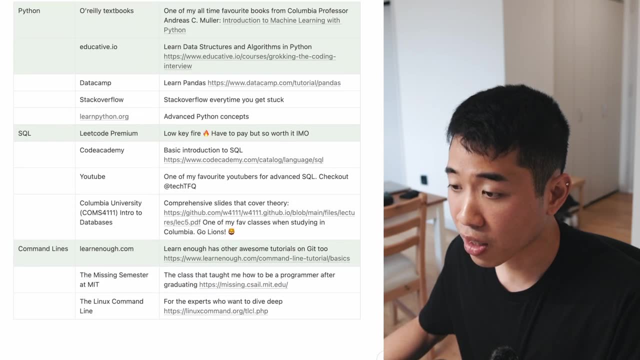 popular ones. I've listed down a bunch of suggested materials. These are by no means definitive, and I'm also going to share a link below, so you don't have to worry about taking notes. I've tried every single material out here that I'm suggesting. The ones in green are some. 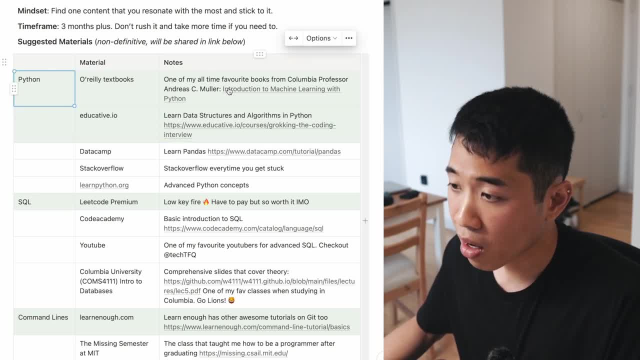 of my personal favorites. For example, this Python O'Reilly textbook on machine learning is not really a Python textbook, but I feel like it teaches Python really, really well. Leetcode Premium was a great resource, although I had to pay for it. 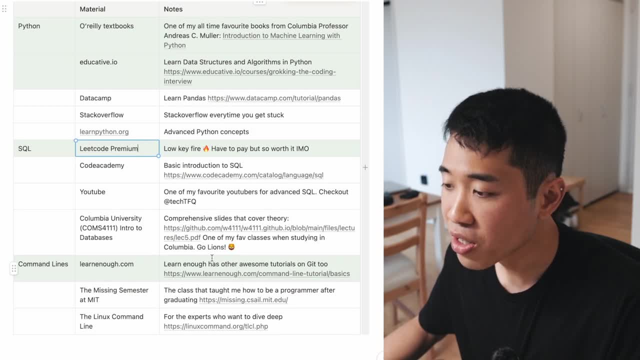 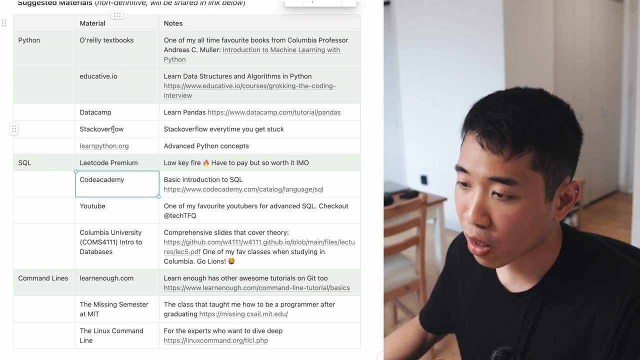 There's this website called learnenoughcom, and learnenoughcom has a bunch of great tutorials. Code Academy is great for getting a high level introduction for SQL. Whenever you get stuck, Stack Overflow is your best bet. Understanding data structures in Python is also one really. 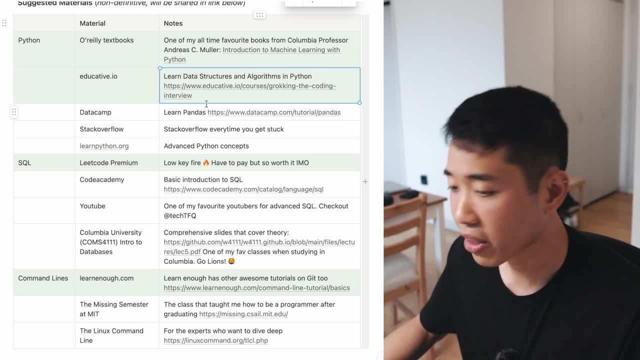 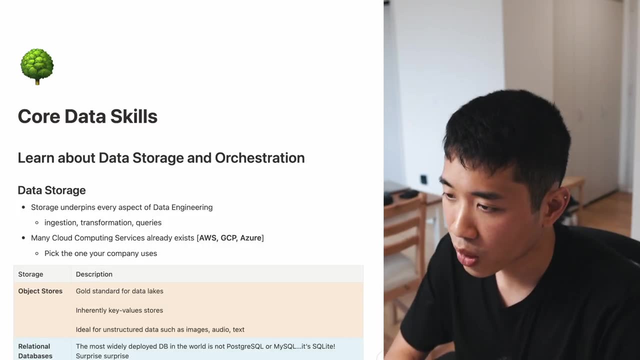 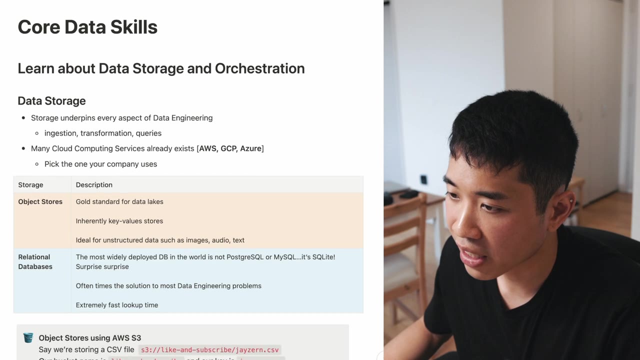 great way to get better at learning the Python programming language. Once you get really good at Python, SQL and Command lines, it's time to learn about data storages and orchestration. Data storage underpins almost every aspect of data engineering, Whether you're trying to perform. 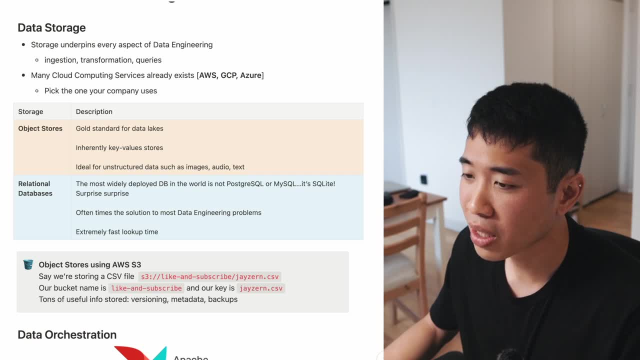 ingestion, transformation or queries. the two most important storage types are object stores and relational databases. Object stores are ideal for unstructured data such as images, audio or text. They're inherently key value stores. Let's say we're storing a CSV file. 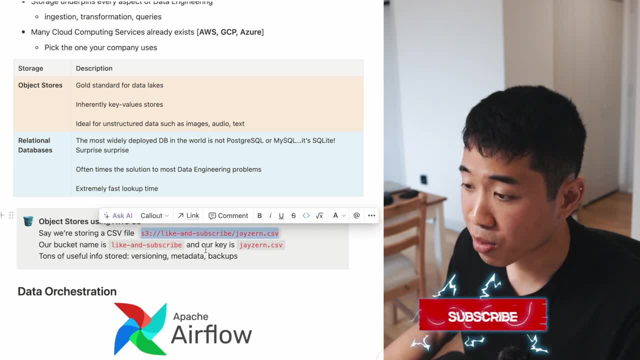 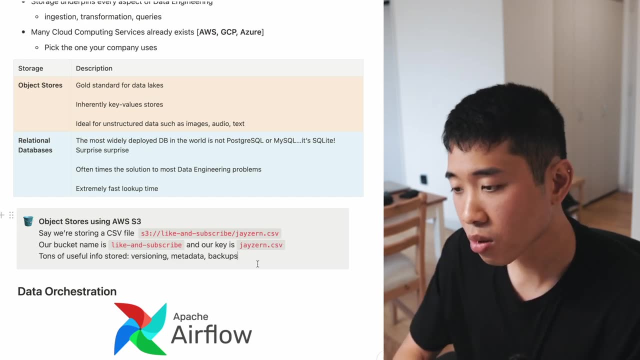 in Amazon S3.. Our bucket name is like and subscribe. Our key is jsoncsv. We're also storing a bunch of useful information like versioning, metadata, data about the data or backups in case something goes wrong. That's what makes the engineering side of things. 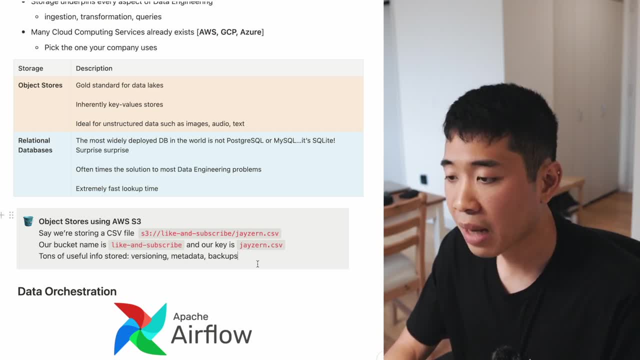 For relational databases. I want to emphasize that it's oftentimes the solution to most data engineering problems. The most widely deployed database in the world is not MySQL, Postgres. Surprise, surprise, it's actually SQLite, Because SQLite has extremely fast lookup times. When you talk about data orchestration, 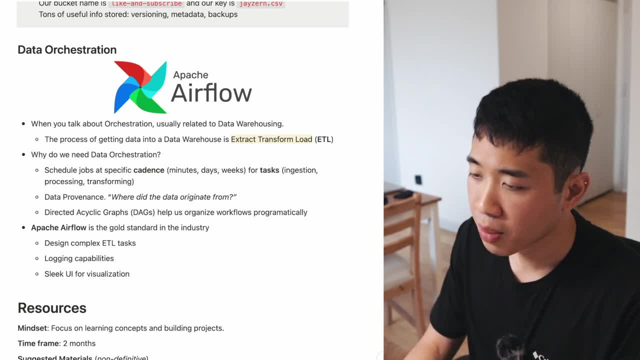 it's usually related to data warehousing. The process of getting data into a warehouse is called extract, transform, load, or ETL for short. You're going to see this term a lot in your career. Why do we need data orchestration? Let's say we're scheduling jobs at a specific cadence for a bunch. 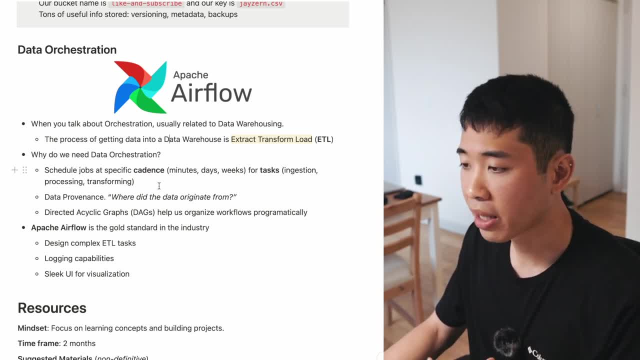 of useful tasks. It could be a daily job in the morning that ingests data into your warehouse. The same thing is that we need data provenance, essentially asking the question of where did the data originate from? Directed acyclic graphs, or DAGs, help us organize workflows more programmatically. 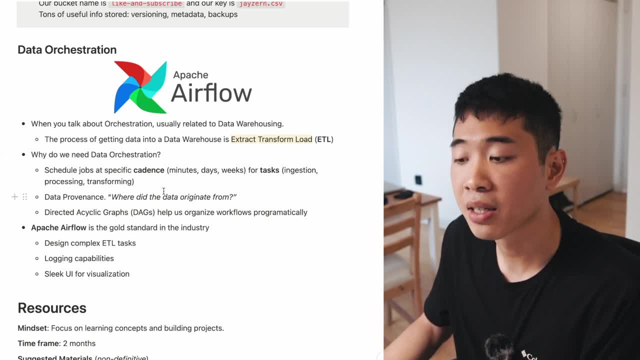 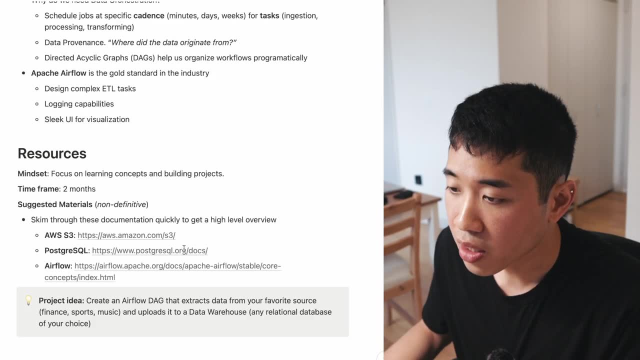 Apache Airflow is the gold standard. I personally really like Airflow because it has great logging capabilities and it has a very sleek user interface to visualize how your DAGs look like. Here are some resources to get started. Focus on learning concepts and building projects. 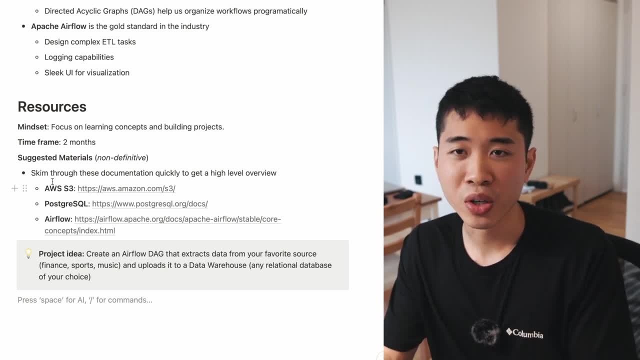 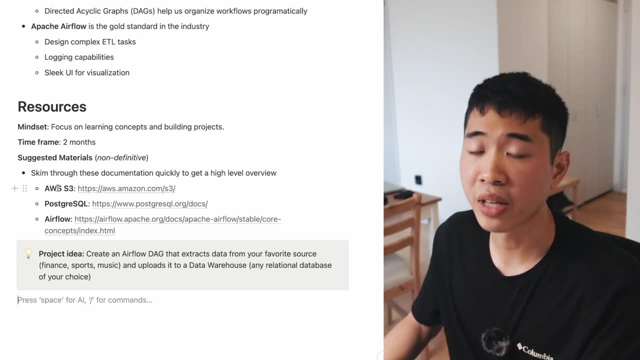 When we learn how to code, we learn how to code. When we learn how to code, we learn how to code. We don't read books to learn how to code. We learn through trial and error and making a bunch of mistakes. I personally would just skim through the documentation of whatever tool that you're. 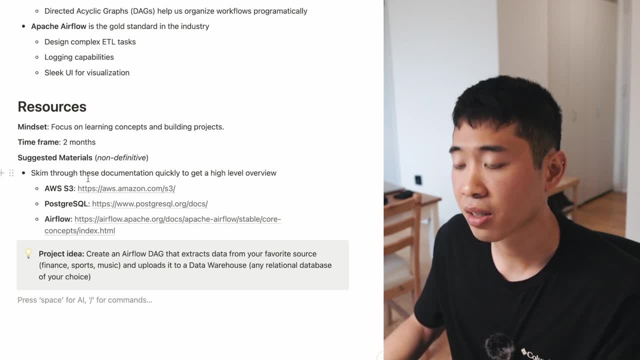 interested in learning and immediately jump on a project. A fun project idea that you can try is to create an Airflow DAG- that extracts data from your favorite source and uploads it to a data warehouse. I think this is a great project to have because it combines your passion and 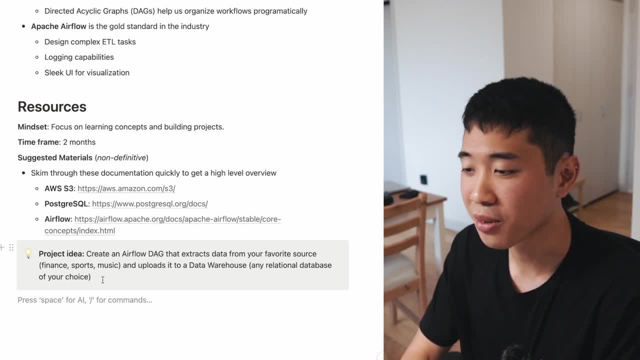 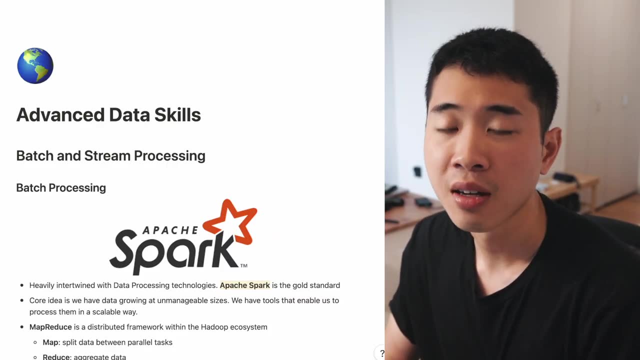 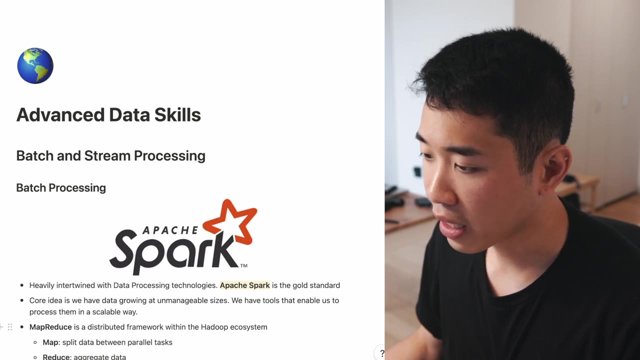 data engineering to create something that you can showcase to other people. Let's talk about advanced data skills, which are batch and stream processing. This is what differentiates traditional software engineers with data engineers. With batch processing. it's often related to big data tools such as Apache, Spark. The core idea is: 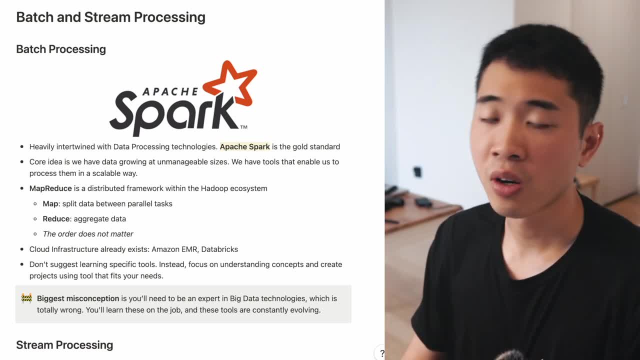 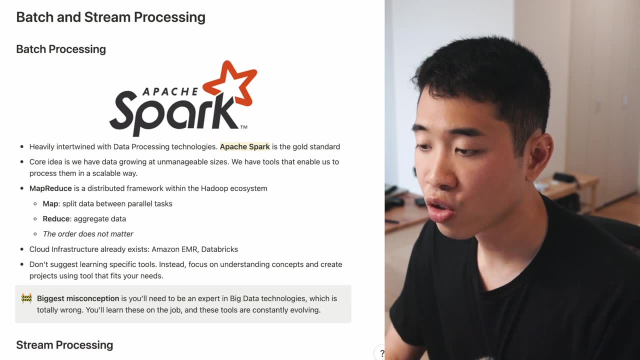 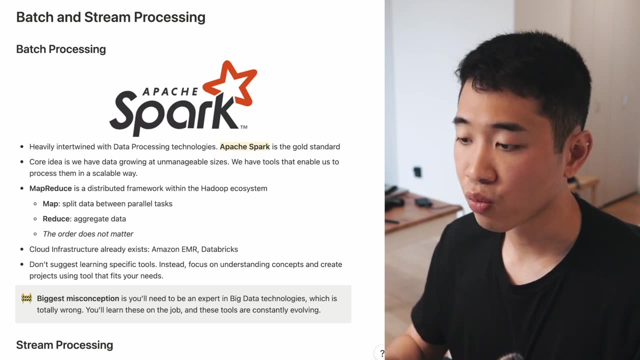 we have data that is growing at unmanageable sizes. In order for us to make sense of them, we built these tools to process them in a scalable way. MapReduce is a distributed framework within the Hadoop ecosystem, where we have a map function that splits data between parallel tasks and a 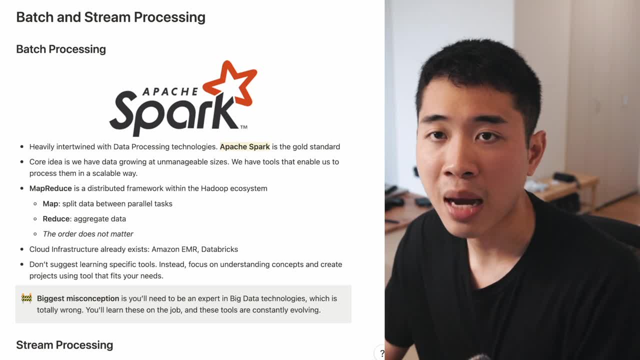 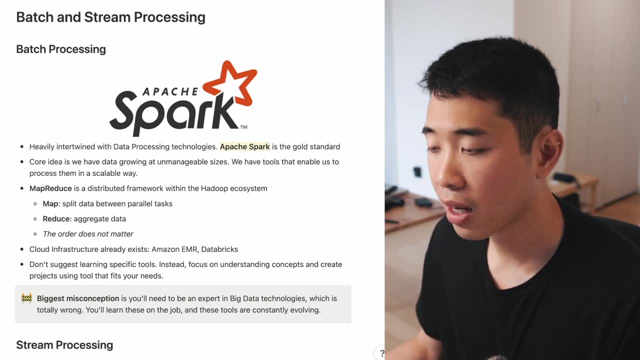 reduce function that aggregates the data. Whenever you see the word MapReduce, I want you to think that the order does not matter. I don't actually suggest learning a specific tool apart from Apache Spark. Instead, I would focus on understanding concepts and create a project. 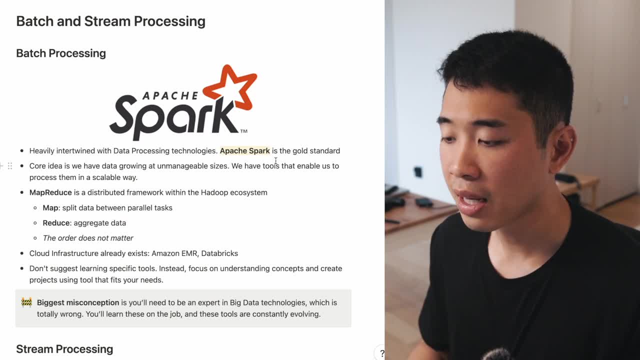 using a tool that fits your needs. One misconception is you need to be an expert in these tools. You will likely learn these on the job. and not only that, these tools are constantly evolving. For stream processing, let's say, we're trying to build a real-time application where 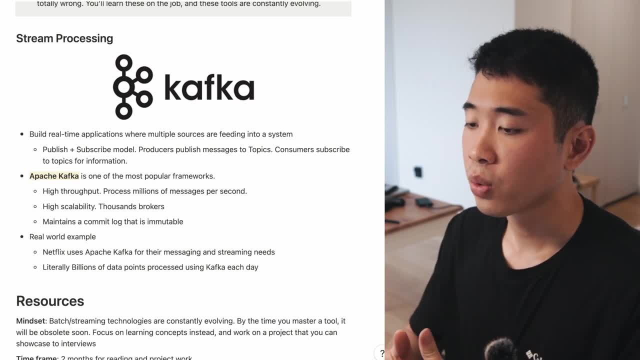 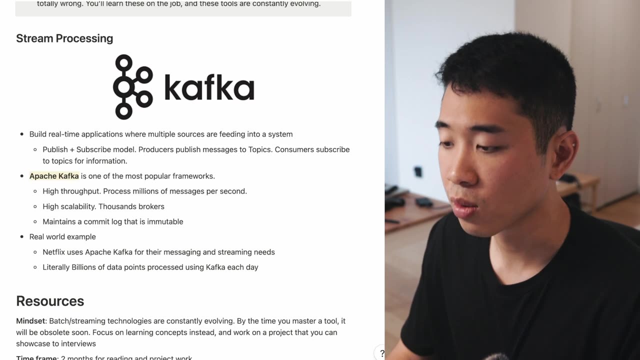 multiple sources are feeding into one system. We have something called a publish and subscribe model, Apache. Kafka is one of the most popular frameworks because it has high throughput, it's scalable and it maintains a commit log that is immutable. One real world example is how Netflix uses Kafka for all their messaging and streaming. 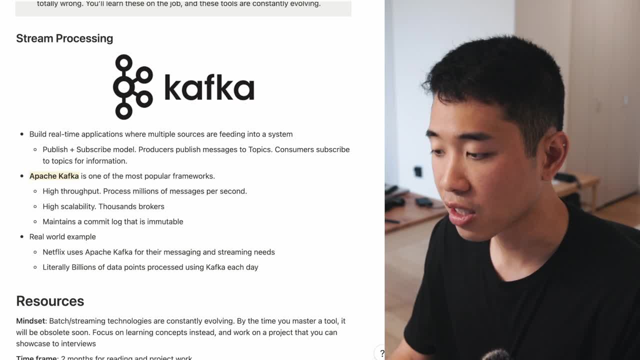 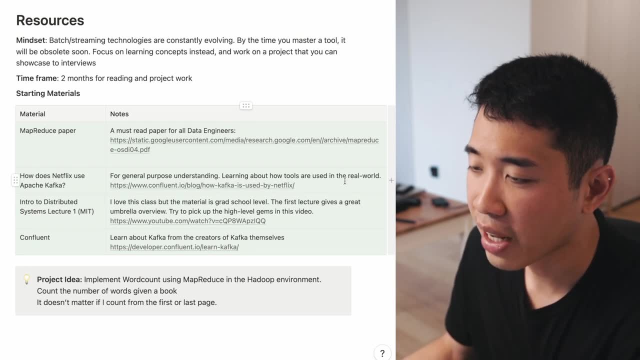 needs. There are billions of data points processed using Kafka each day, and that's how important stream processing tools are. Here are some resources. I want to caveat this by saying batch and streaming tools are constantly evolving. By the time you master one tool, it's going to be. 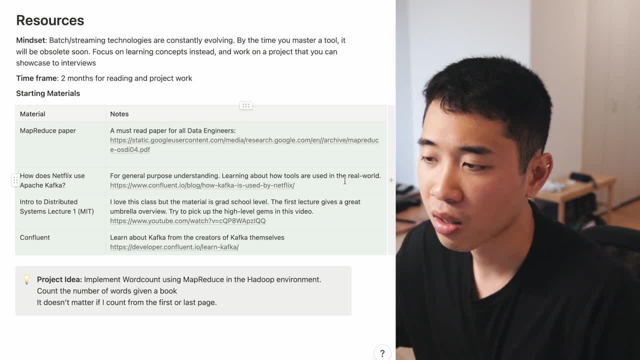 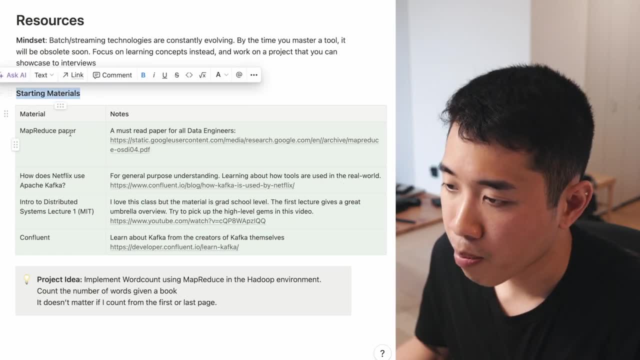 obsolete very soon. I would actually focus on learning concepts instead and just work on a project that you can showcase to your friends or your interviewers. I feel like this MapReduce paper is a must-read for all data engineers If you're interested in learning more about. 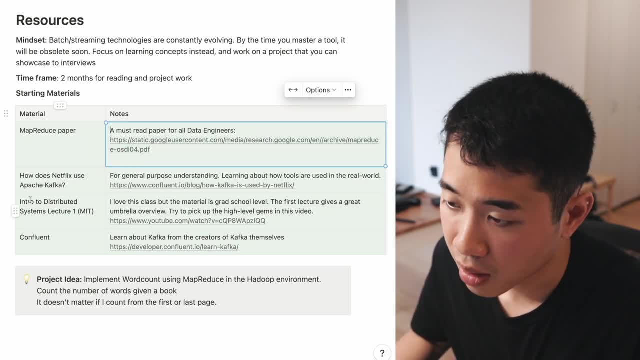 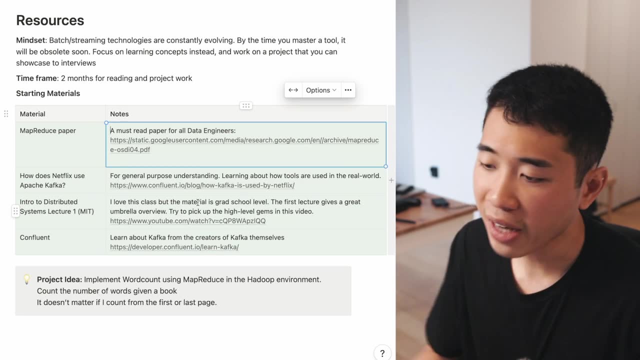 distribution systems. this class Introduction to Distributed Systems. the first lecture gives a great umbrella overview. Try to pick up some of the high-level gems in this video. Here's a practical project idea: Implement word count using MapReduce. Let's say I'm trying to.